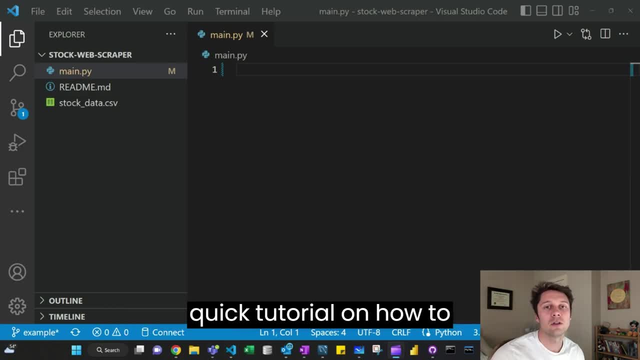 Hi everyone, my name is Brandon and today I'm going to take you through a quick tutorial on how to web scrape a stock market page. So we're going to start off with this mainpy file. That's going to be our main file where we run our code. We'll start off by importing a library called requests. 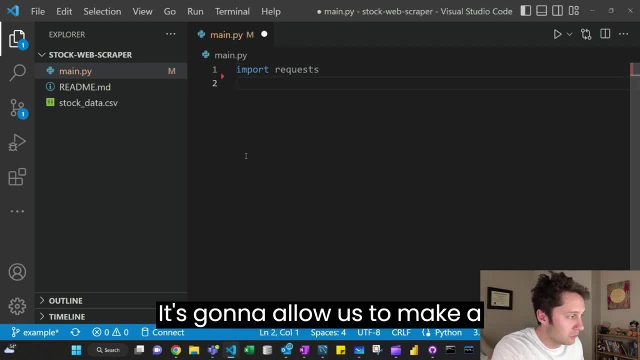 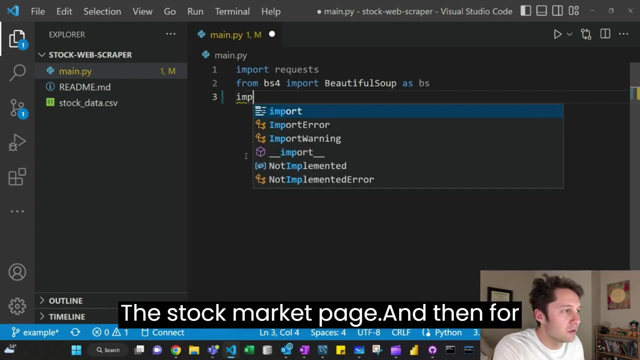 This is going to allow us to make a request to a server and get a response from the stock market page And I'm going to say from BS4: import beautiful soup, Yes, And this is a tool that's going to allow us to parse the HTML code on the stock market page And then, for performance, 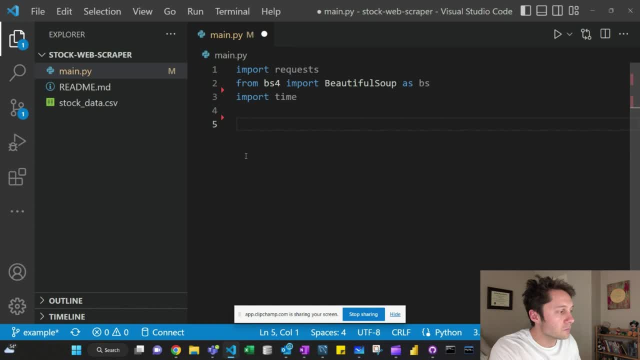 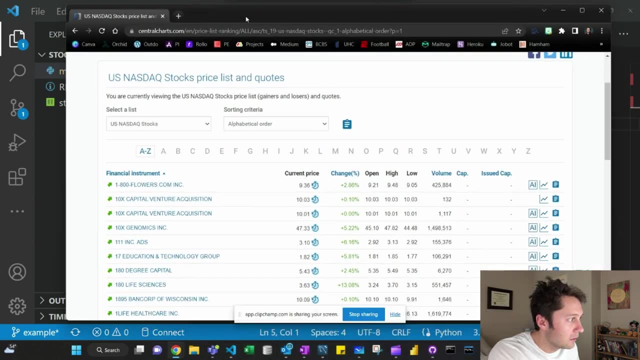 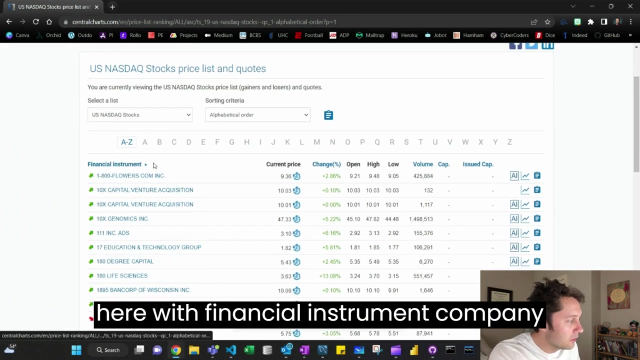 testing, we'll import time. So, for reference, the stock market page that we're going to be looking at today is this one at centralchartscom And, as you can see, we have a table down here with financial instrument company name prices. 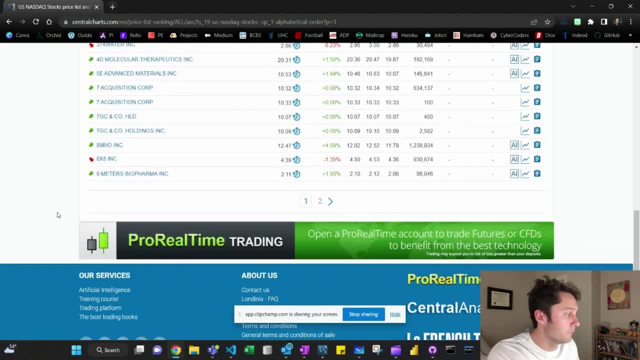 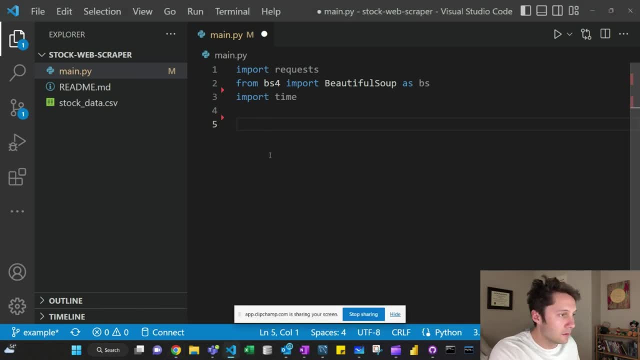 percent change where it opened the high, the low, et cetera. So if we go back to the code, we'll start off with declaring whatever. we start with the time. We're going to start off with declaring the time whenever we start the code. 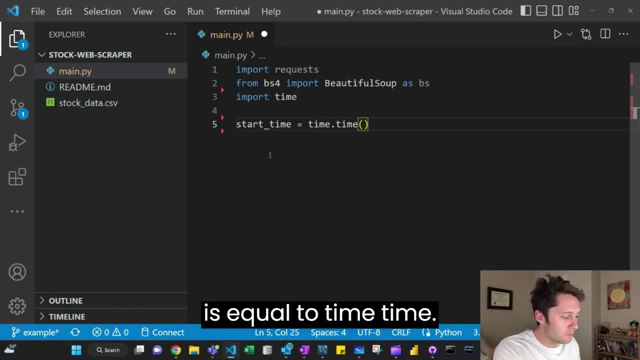 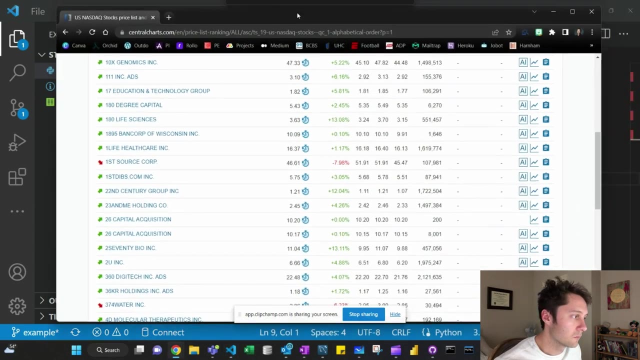 Start time is equal to time dot time. Whenever we run the code, it'll mark whatever time we started. Now we're going to create an empty list where we're going to store all the pages. So we're going to create an empty list where we're going to store all the pages. 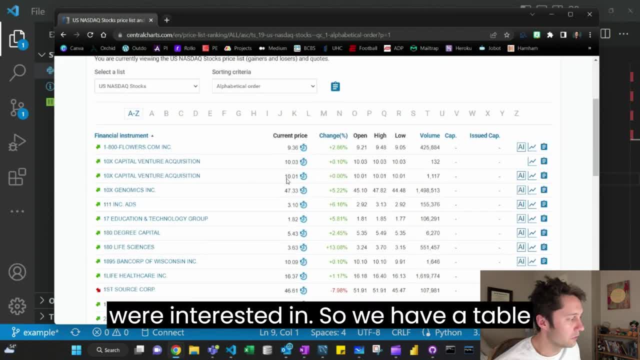 And we're going to create an empty list where we're going to store all the pages on this website, at least the ones that we're interested in. So we have a table of stocks here And you can see there's multiple pages if you scroll down to the bottom. 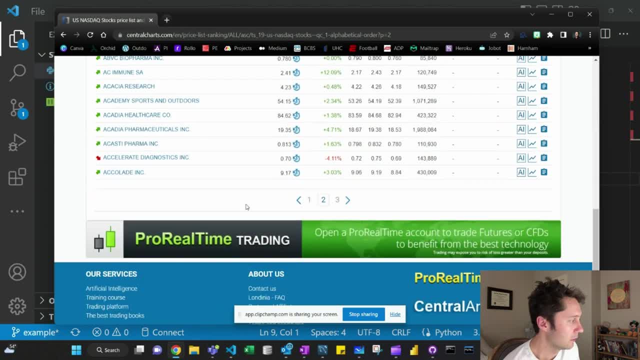 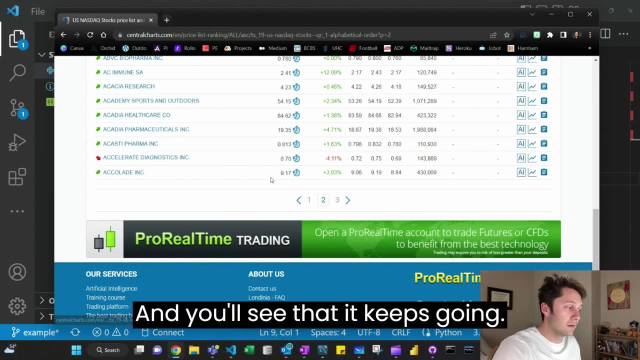 So we click on this one. Here's another list of stocks and it's in alphabetical order, And you'll see that it keeps going And if you look up at this URL: centralchartscom, centralchartscom, centralchartscom. 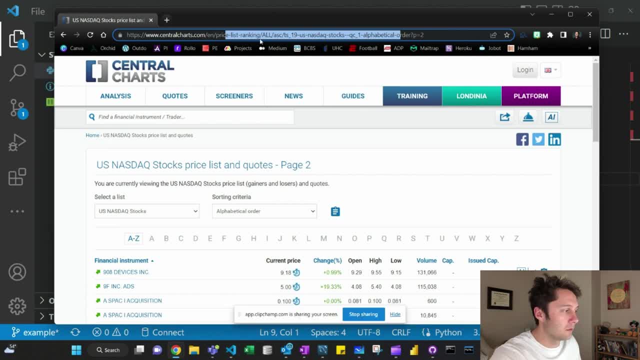 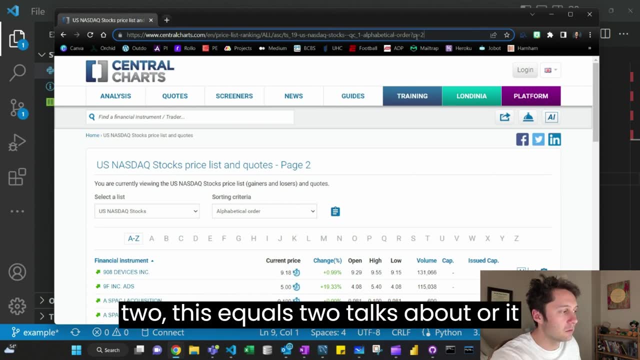 centralchartscom, centralchartscom, centralchartscom, centralchartscom. and then there's some other information within the URL here, But then at the end it says p equals 2.. This p equals 2 talks about, or it tells you what page you're actually on. 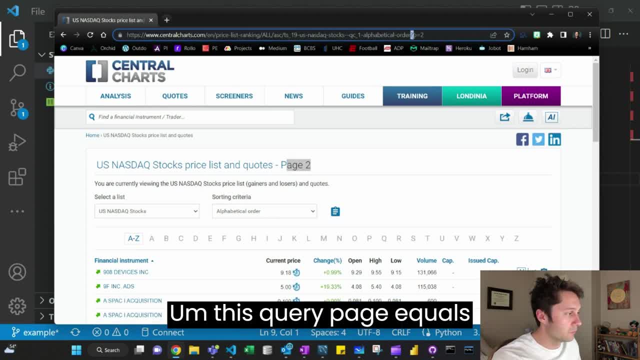 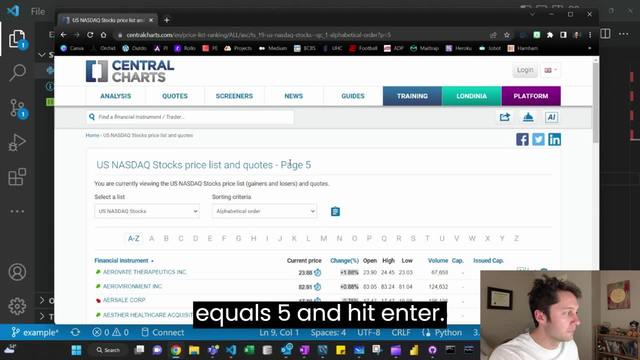 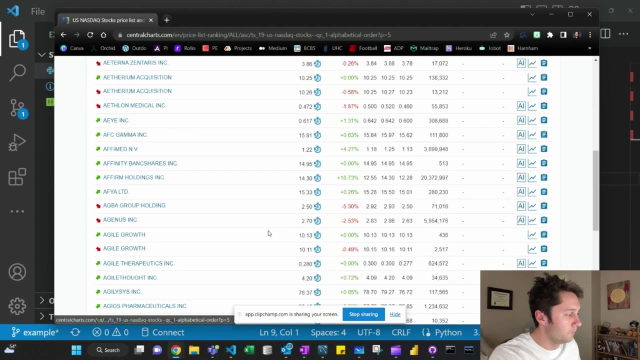 So, because we're on the second page, it says query page equals 2.. So if I change this URL to p equals 5 and hit enter, it'll take me to the fifth page of the stock market summary, And then it'll take me to the fourth page of the stock market summary. 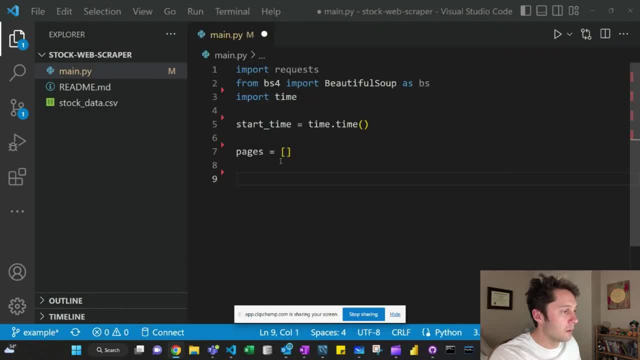 So what we want to do is take all these URLs, put them in a list that we're going to call pages, and then we're going to tell our program: OK, go through each URL in this list. request the information from the server. 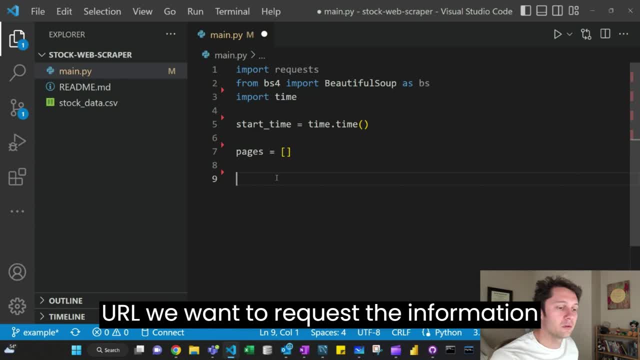 telling it for that URL. We want to request the information from the server and then from there we can parse the information. So we can say, OK, let's do that. So we're going to say, OK, let's do this. 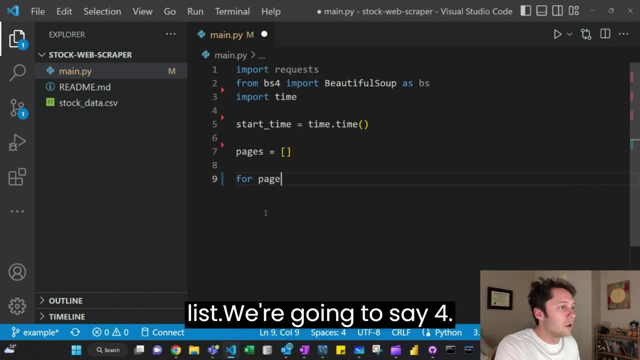 So, starting off with this empty pages list, we're going to say for page number in range, And for our example, let's just say we're only interested in pages 1 through 4.. We'll say: URL start equal to URL start equal to. 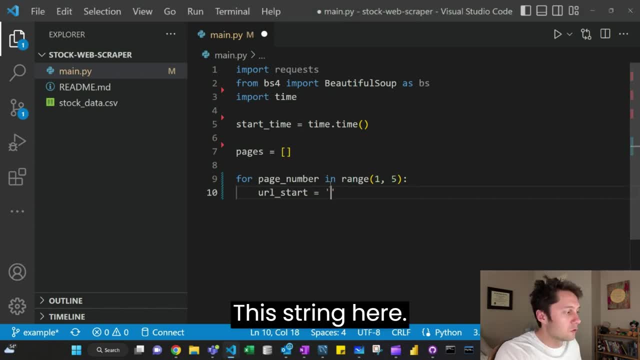 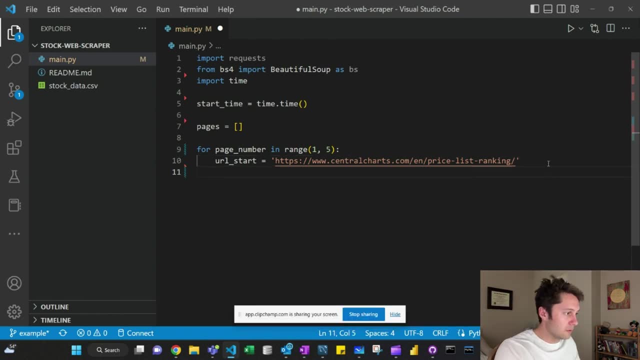 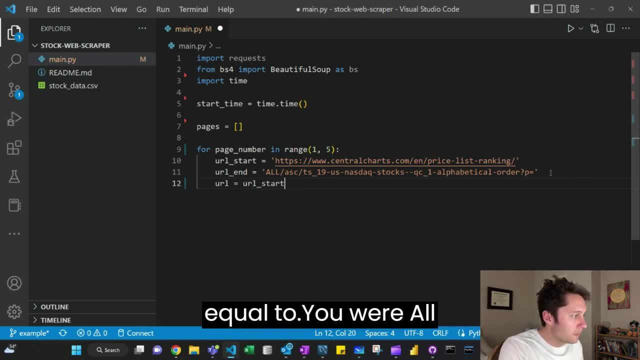 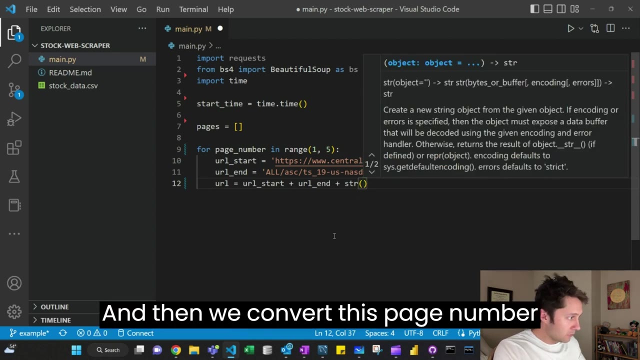 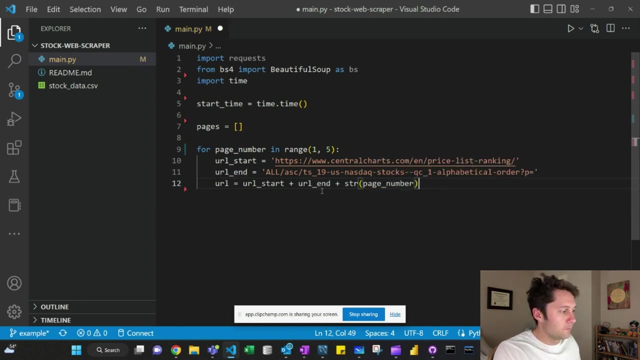 And then I'll say URL is going to be equal to URL start plus. And then I'll say URL is going to be equal to URL start plus URL end plus. And then we convert this page number that's in the for loop into a string. And then we convert this page number that's in the for loop into a string. 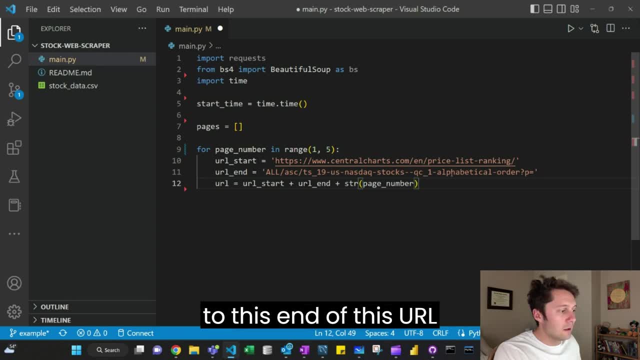 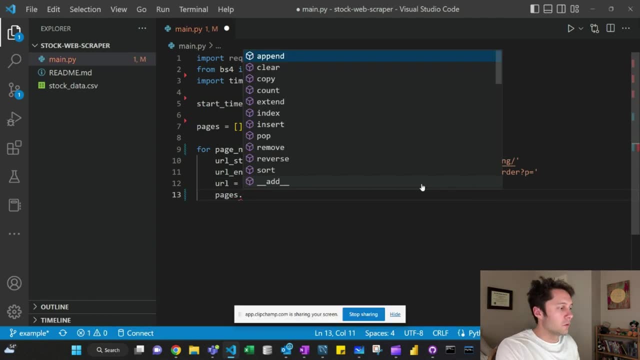 So that we'll just add this, pop this on to this end of this URL end string. So once we have this URL, So once we have this URL, So once we have this URL, We're going to say pages dot- append URL. 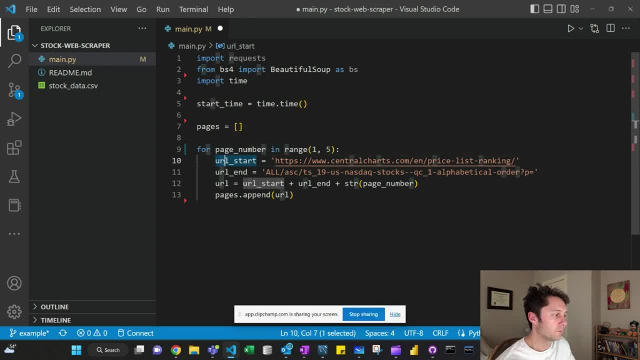 So for each page number going one through four, we're going to take the beginning of the URL, the end of the URL and that page number, We're going to create the URL and then we're going to add it to this empty list up here. 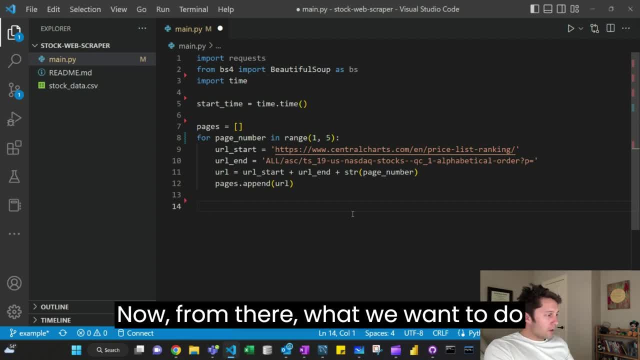 Okay, Now, from there, there, what we want to do is: so we'll have this list of URLs, and what we're going to want to do is request from the server. we're going to say, hey, I want the information from this URL and we'll get a response from that URL, so we're going. 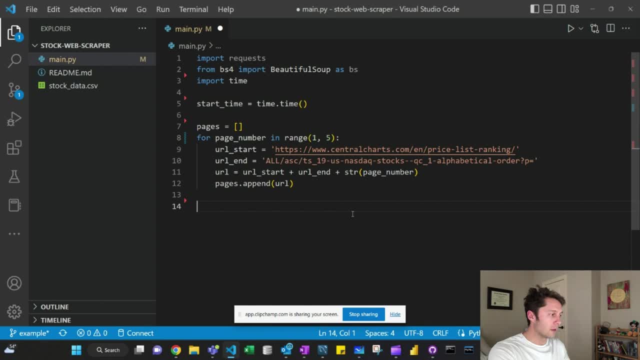 to use the requests library that we already imported before but to store the response, we're going to first create an empty list. so let's say values underscore list is equal to empty list. now we're going to say for page and pages: for each page that's in the pages list that we have, that we've already created. let's: 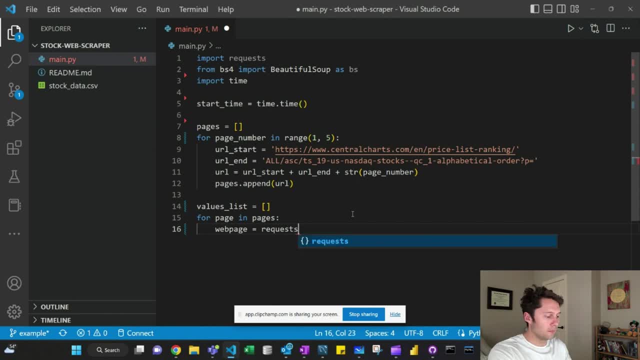 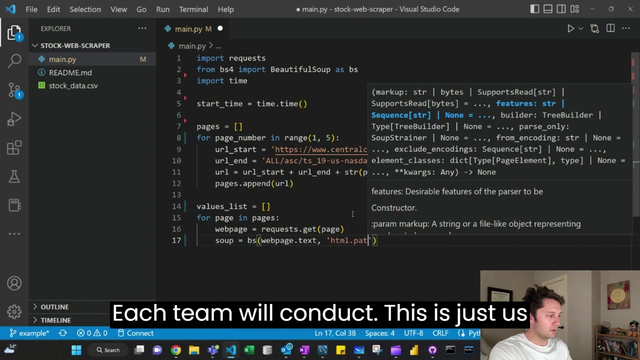 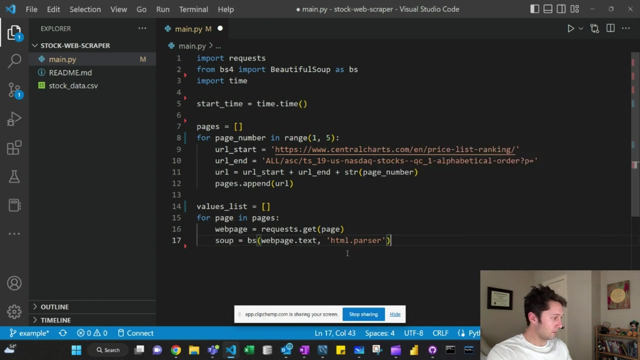 say: web page is equal to lists dot age. and now to set up the beautiful soup HTML HTML parser, we're gonna say: soup equals BS. web page text HTML. this is just saying: hey, get the response request and then we're gonna. we want the text from the your page that we just received. 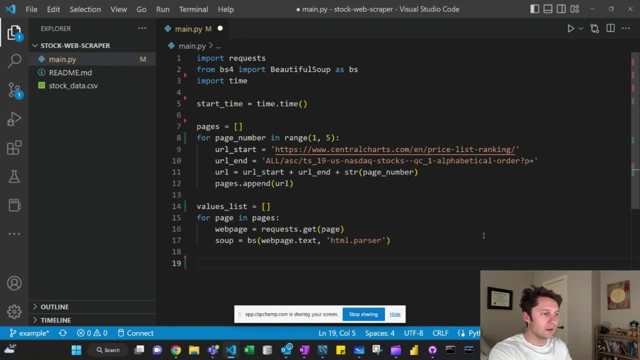 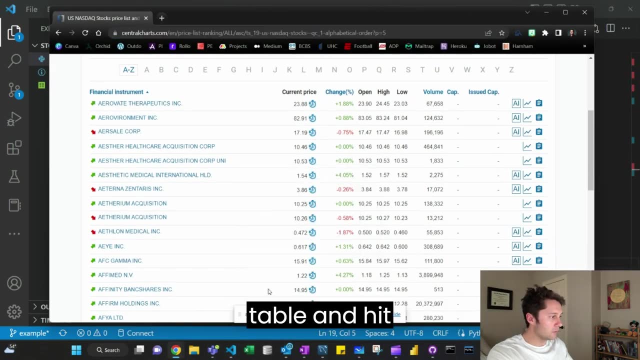 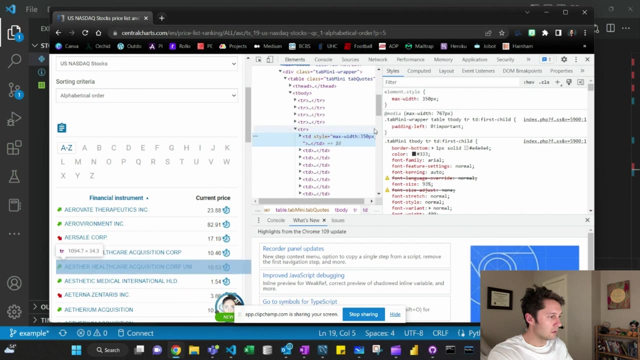 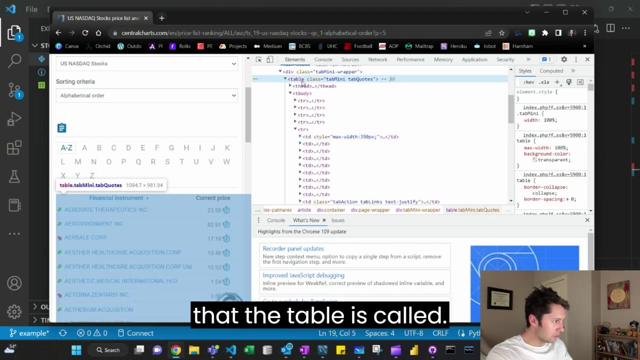 so let's go back to our stock market page. so if you click on the table and hit inspect, right right click on the table, hit inspect. let's move this over a little bit so that you can see it. you'll see that the table is called. the table has a class called tab- mini space- tab quotes. 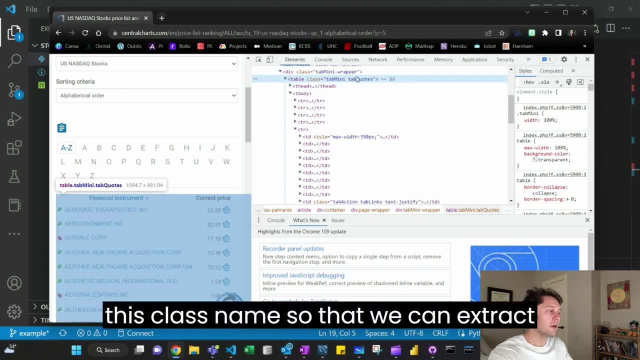 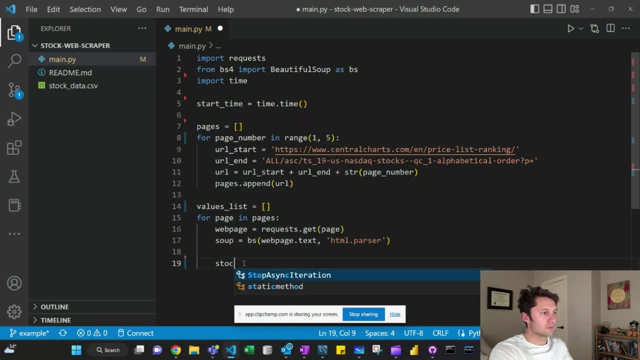 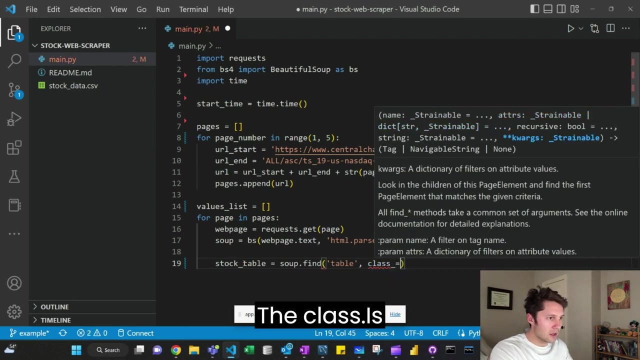 so we're going to actually reference this class name so that we can extract the table information. so we're going to say: stock table is equal to soup def find. I mean the table, the class is named haveMany haveQuotes. All right, so now we're going. 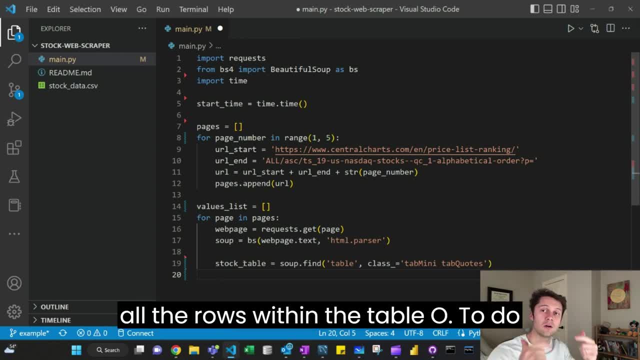 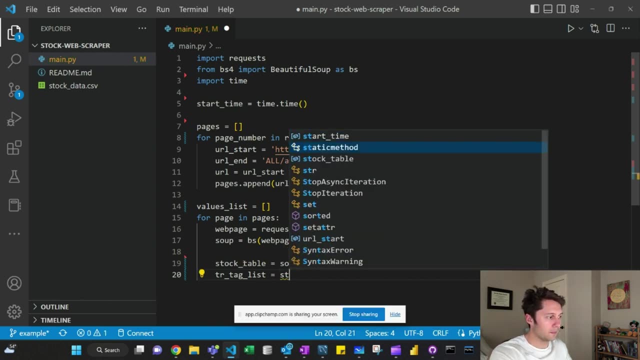 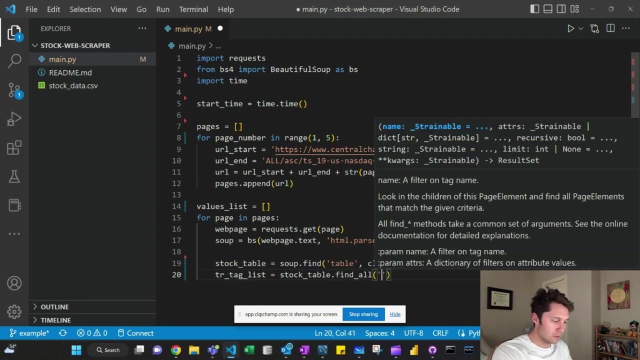 to cycle through that table and try to find all the rows within the table. So to do that, we're going to say tr- underscore tag. underscore list: tr tag list. We're going to make a list of all the rows Table: find all, find all tags labeled tr. 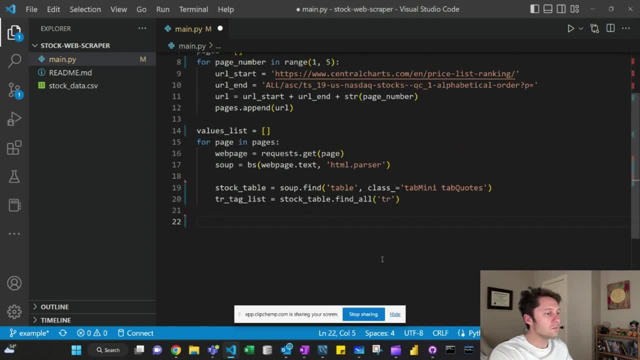 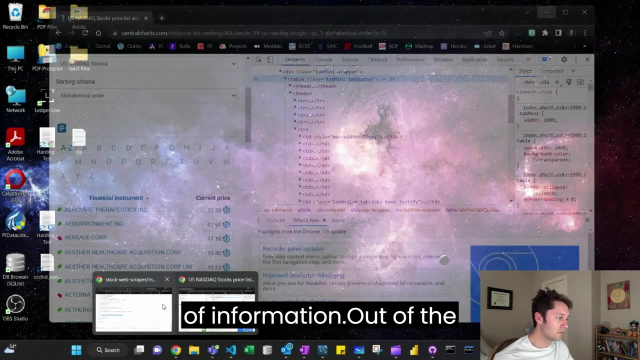 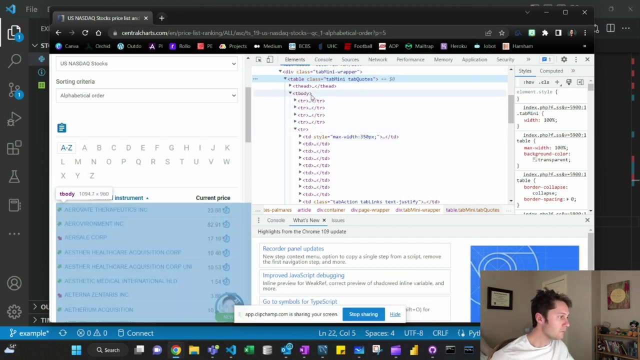 All right, And now, within each row, we want to find the td tags, the table data tags, so that we can actually pull the individual pieces of information out of the table. So if we look back at our table, we have table. we have each row and within a row, each. 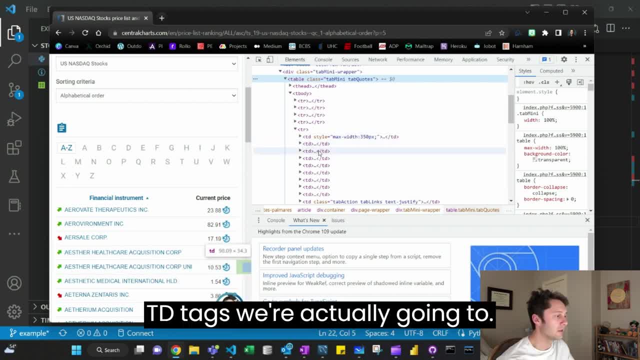 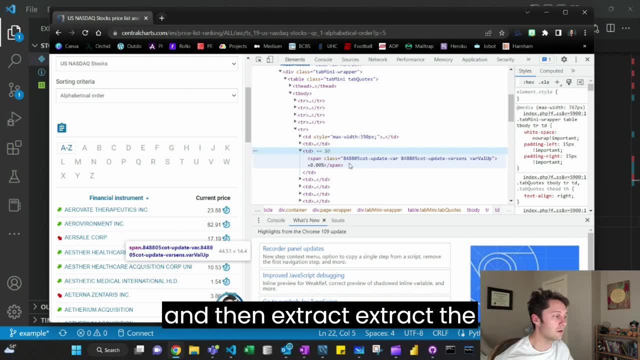 table cell And then the first row we'll show is Within the row In the column. so this first row is going to show our ч for the time being. So we can't, let's say we can first try this one. 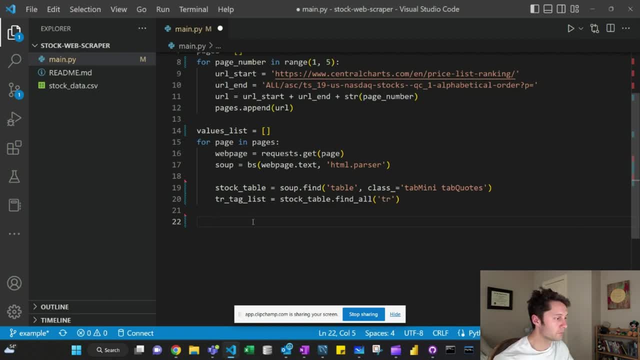 maybe something else, but just to let you know that the summary column is defined by this: td tags. we're actually going to, Our program is going to find the td tag and then extract the information from it. So to do that, we're going to say for each tr tag in tr tag list: 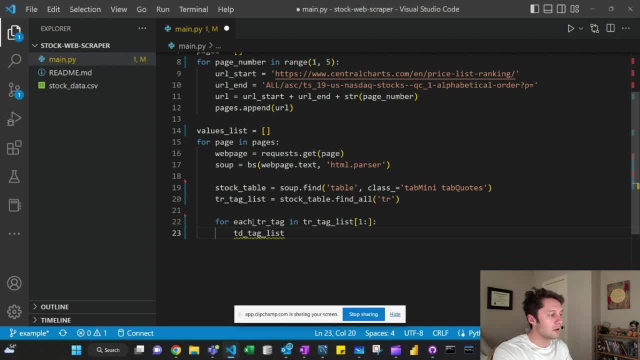 I'm going to say td underscore tr tag list. tag list is equal to each tag and all TD. so we're making this TD tag list where each TR tag move on within each TR tag. we want to find the TD tags. now let's create another empty list to store the TD, the labels for each TD tag. you can say: 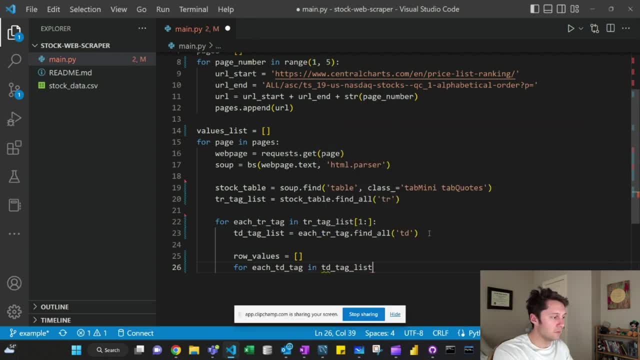 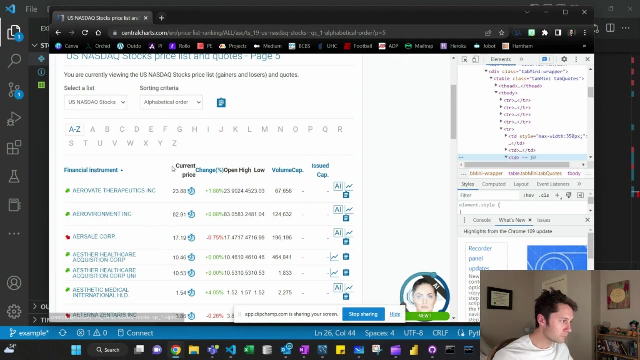 for each key tag, the key tag list. let's just get the first. let's just get the first seven. if you look back at the URL, if you look back the web page, really it's just the first, like one, two, three, four, five, six, seven, seven. the seventh column is this: 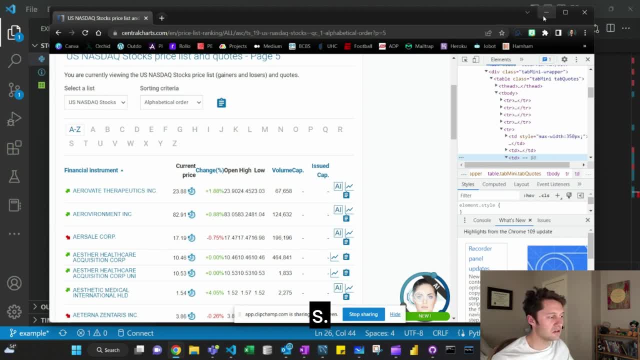 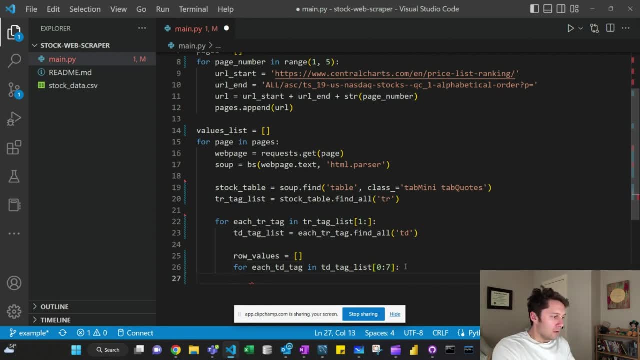 volume one. after that these are blank or just not that important. so we're just going to get the first seven columns. then we can say: new value is equal to each TD tag text up, strip and get the text in the proper format. now we're gonna say row values, append new value. all right, now we're gonna have this. 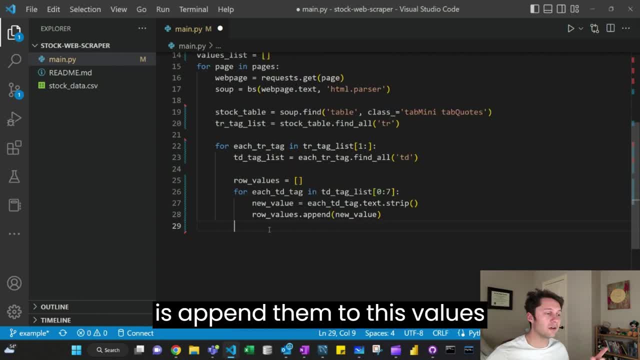 list of the row values, and what we want to do with those row values is append them to this values list, and then that's what we're going to print out so that we can see all the information from the web page. so what we're going to do now is just say: values list, append- we're going to append this row. 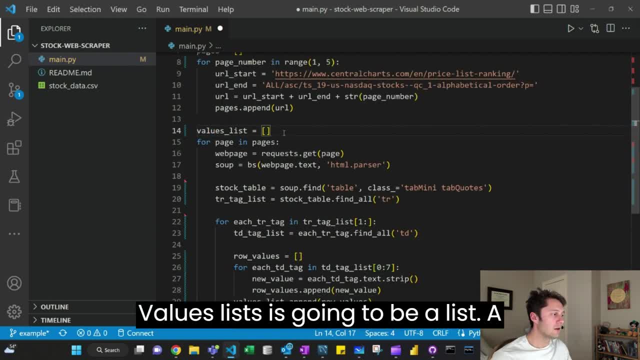 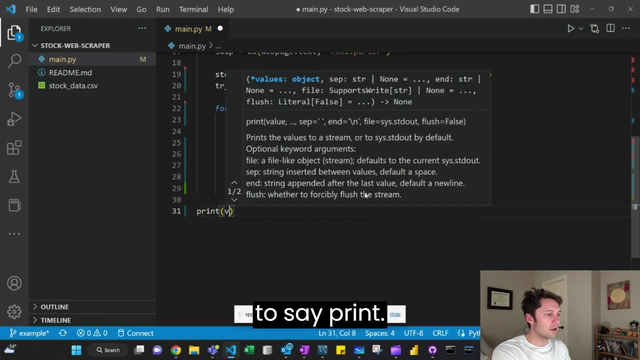 values list that we just created. so we're going to create a list of lists. values list is going to be a list that contains a bunch of lists and those lists will represent the information within each row within the table, and that's it. so now we're just going to say print values list, so we can. 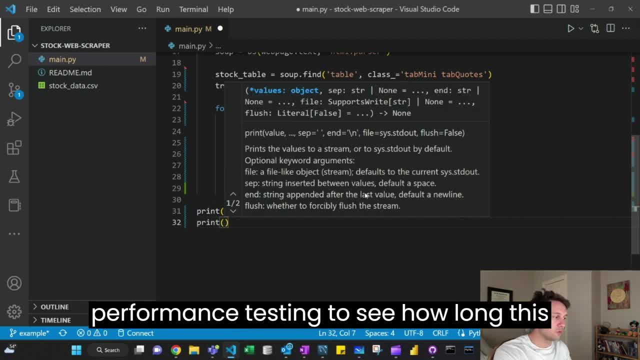 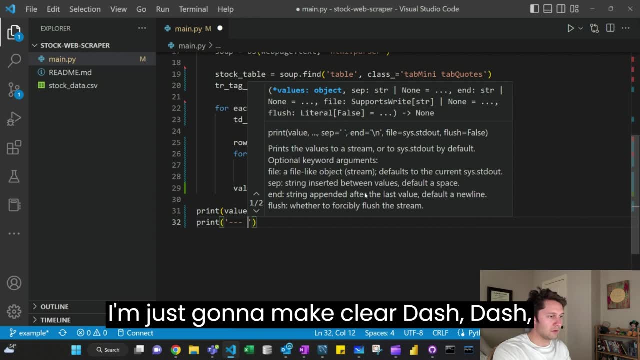 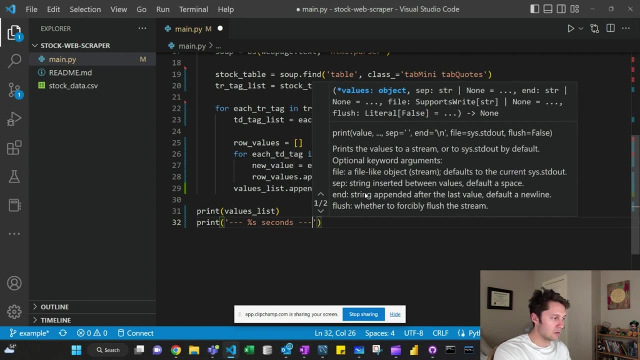 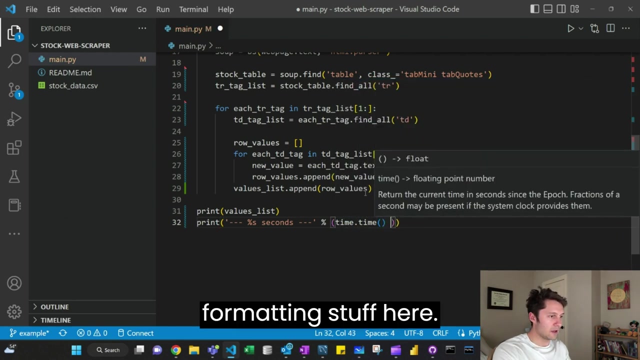 see the information and to finish off our performance testing, to see how long this takes, let's just say print um. i'm just gonna make it clear: dash, dash, dash um s seconds percent formatting stuff here. time time is the current time minus the time that we started, which. 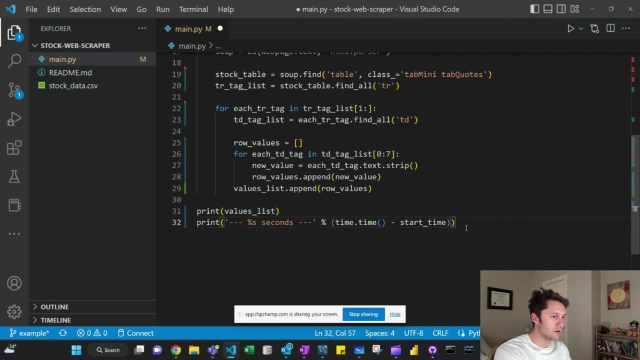 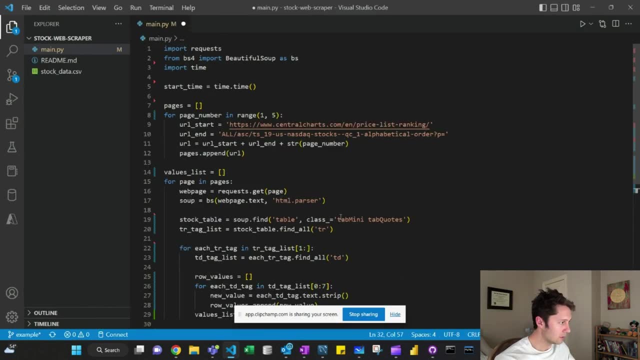 we've already defined. okay, and that should be it. so let me, let me zoom out here so you can see the whole thing. so first, we created this pages list to um, you can see that we've already created this page list and we're going to go ahead and do that. 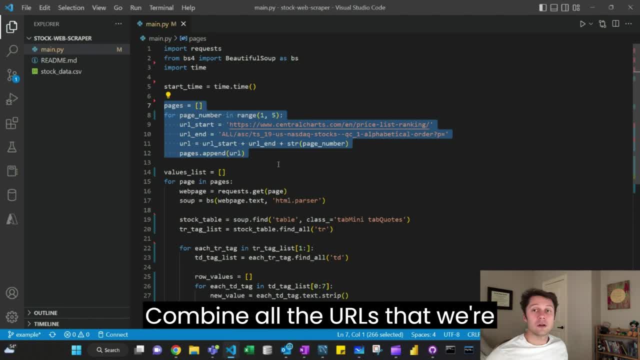 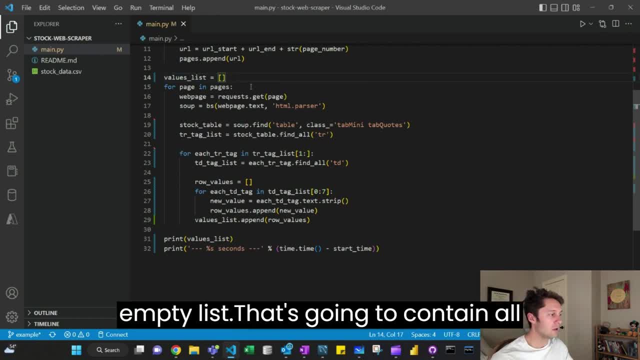 and then we're going to create this empty list that's going to contain all the information that we've, that that's included in the response from the server, and then these: the series of for loops goes through each page, each row on that page and each td tag within each row. 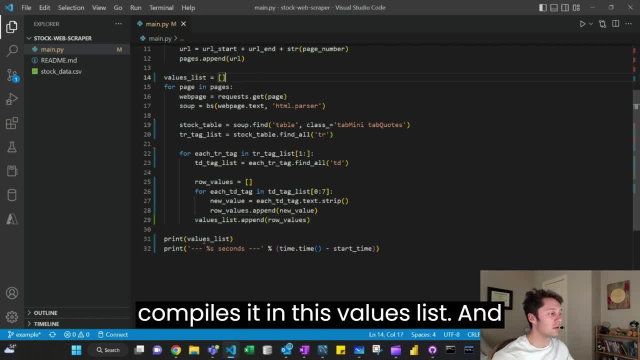 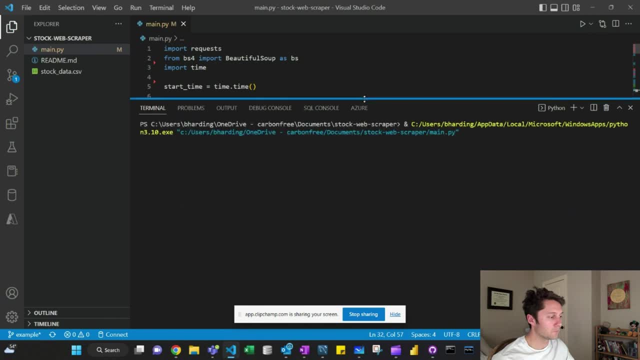 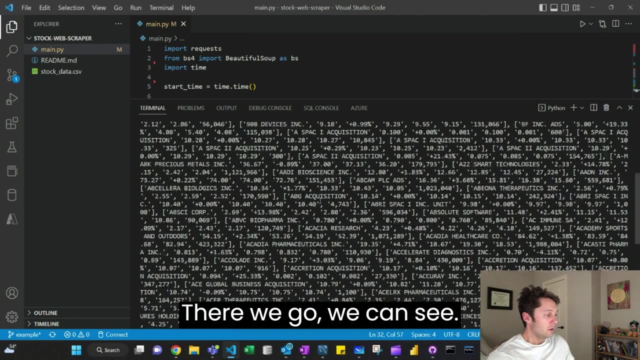 extracts the information and then compiles it in this values list and then we're going to print the list and then see how long it takes us. so we're just going to run this here and then if we look up and look down at the terminal, there we go, we can see. 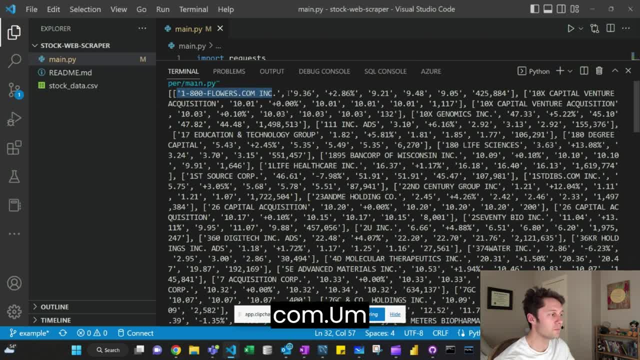 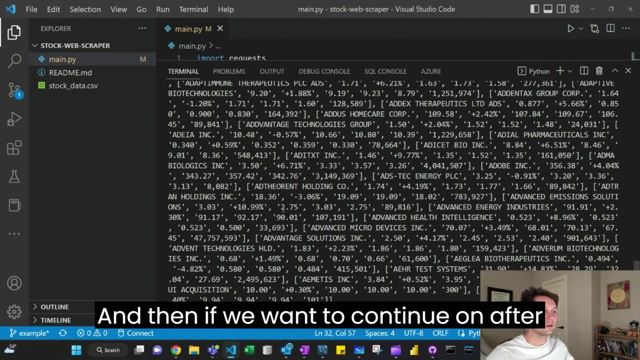 we can see that 100flowerscom- um is our first. um is our first list within this list, and each of these represents the information within that row and then each list after that is is rep, is one row and then, if we want to continue on after this, we can. 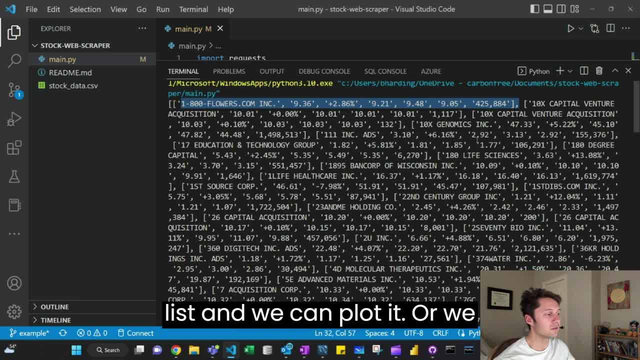 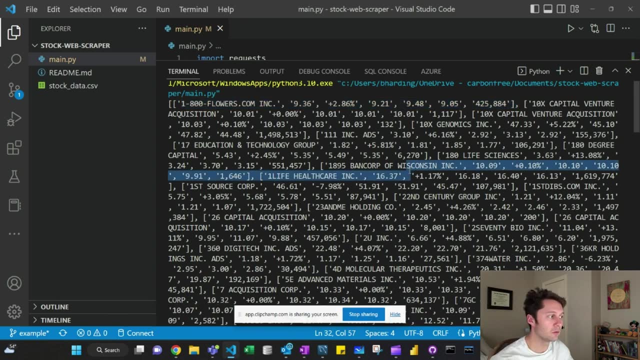 you know, pull the information out of each list and we can plot it or we can analyze it further, whatever you want to call it. but we can also do this in the same way we want to do. but, um, the hard part is getting it in this format. so what i think is pretty cool is that we were able to cycle through five pages, and you can.